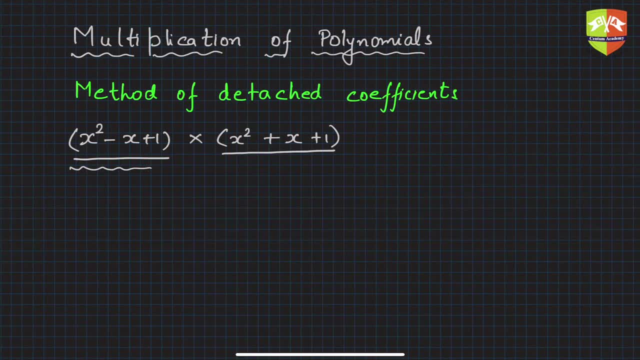 if you see the first factor or the multiplicand. in this case the degree is two. So hence powers of x is one- sorry, zero- one and two. So you can see it is completely written like that. So power of x is zero, then one, then two. Similarly, here also it is complete polynomial, because all the powers of x 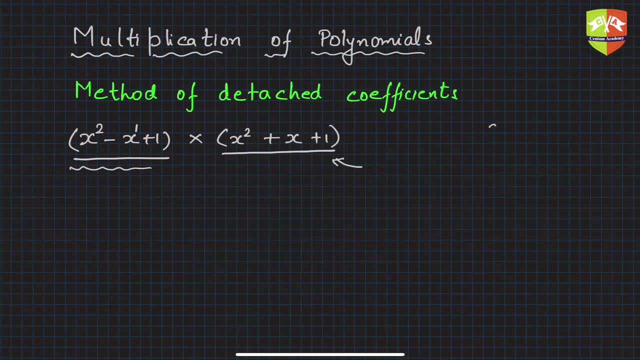 are reflecting over there. Now, let's say, if you had an expression like x cube plus one, okay, and one of the multiplicands would have been this, Then you have to write it like x cube plus zero times x, squared plus zero times x, and then finally one right. So this is the 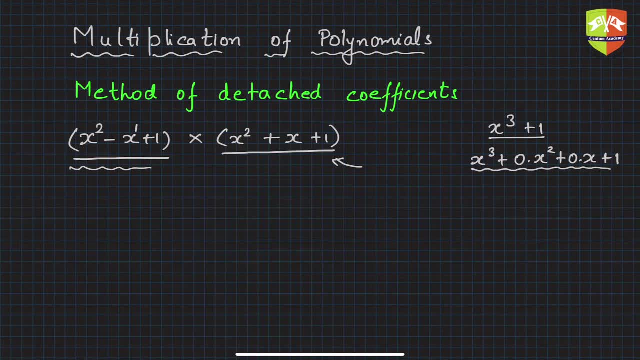 complete polynomial. Now, once you have written the polynomial completely, that means all the powers of the variables have been expressed- then you need to just detach the coefficient. So you know all the coefficients which you can see. So let's take the first polynomial here: x- square. 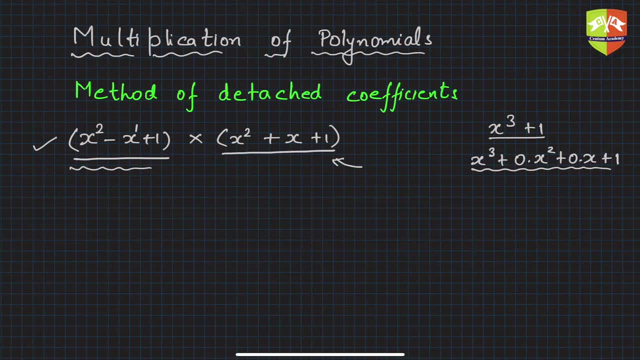 minus x plus one, this one. The detached coefficients will be simply one minus one and one, So I'm writing it like that, okay? Similarly, in the second case, it is one plus one. So you can see that it is one and plus one, isn't it? So this is what it is Right now. we have to just follow the normal. 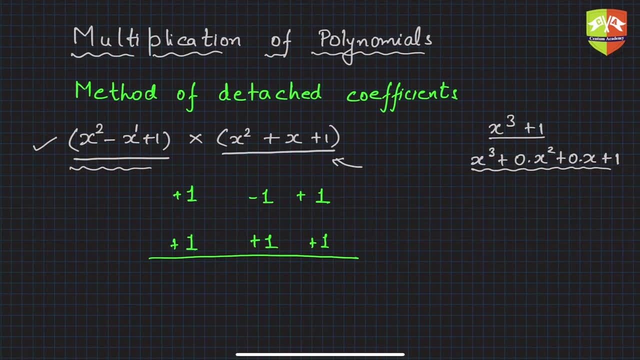 process of multiplication. You know the way we do multiplication Now. first thing is, multiply this one by plus one. So what is the result? You will get plus one. Okay. then multiply this by this. You will get minus one, and then, finally, this by this. So what do you get? You get plus one again. 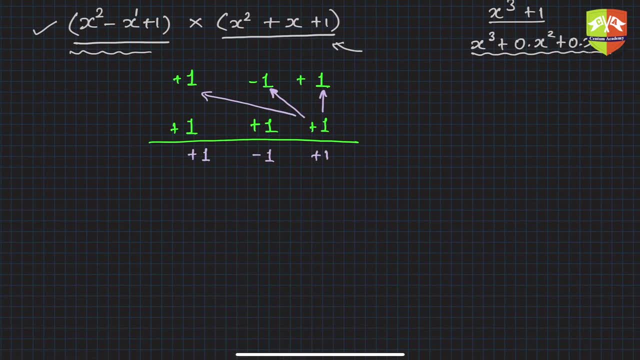 Now for the second line. what you need to do is now you have to take this one and multiply with this one and write just like you shift in your normal multiplication process. So you will write plus one here, Then this one will get multiplied by this minus one here and the product is minus one, just right in. 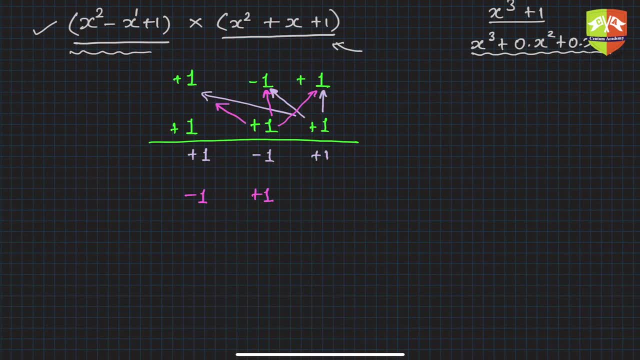 the left of it, And then finally this one. So this will be plus one. Okay, now, you would have guessed it by now. So what do you need to do next? Take this one and multiply by right and write it here. The next one, you know So exactly underneath this one. So 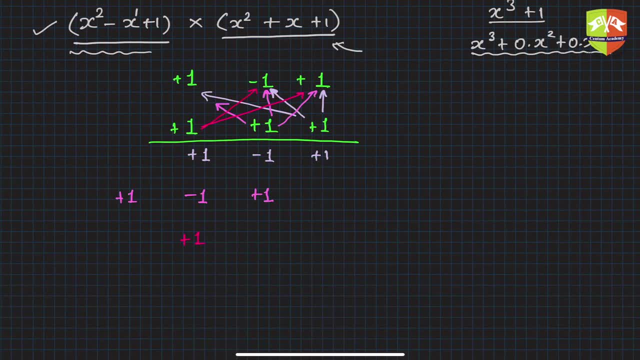 this is plus one And then right, So multiply that, You'll write minus one and this here, You write plus one here, And then finally you sum them the way you do it in normal multiplication. So this is one. clearly, this one is zero, this one is plus one. again, this one is zero and this one is plus one. 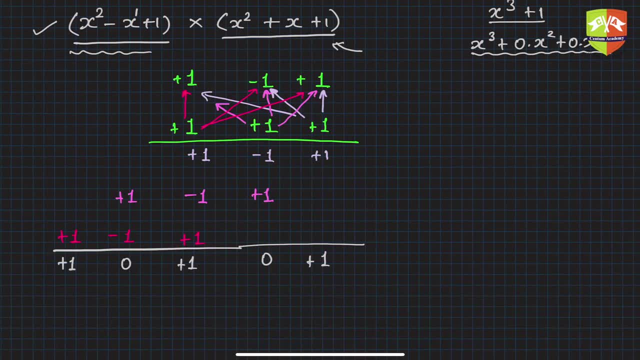 again. and now you know how to the. what is the final result? so you have to just start putting the powers of: or. the x is here, so x to the power zero, x to power one, x to power two, x to power three and x to power four. right, so the product is simply x to the power four plus x, square plus. 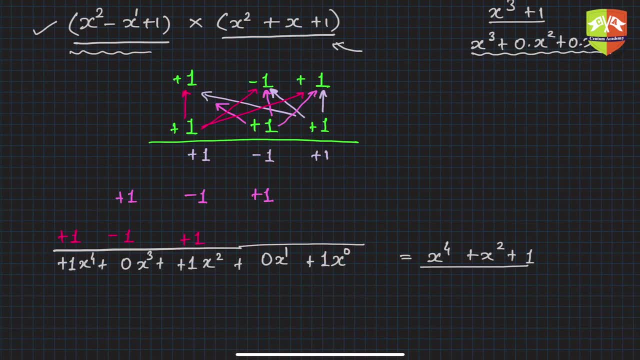 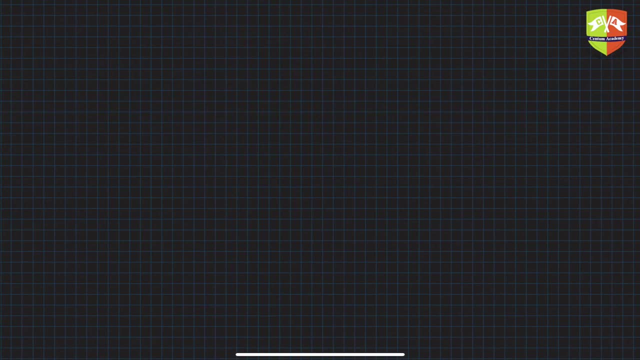 one. you can check that this is the product. okay, let's take another example to make it more clear now. let's say we have been given two polynomials. one is x to the power, five plus x, cube minus two, x square plus three. okay, this is polynomial number one and it has to be. 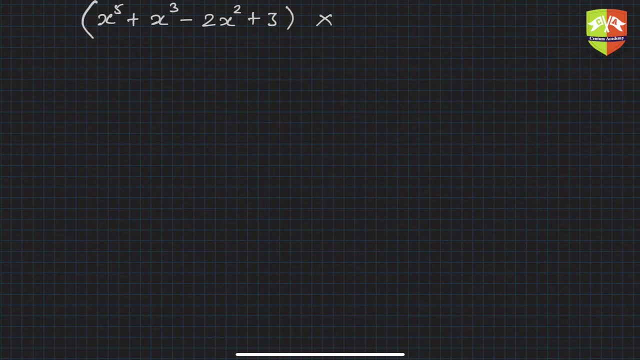 multiplied by this: one, two x to the power four minus three, x cube plus four, x square minus one. okay now, if you can, uh, you see closely. these two polynomials are not complete. there are few powers of x which are missing, so let me, you know, complete the expression. so it will be x to the power five. 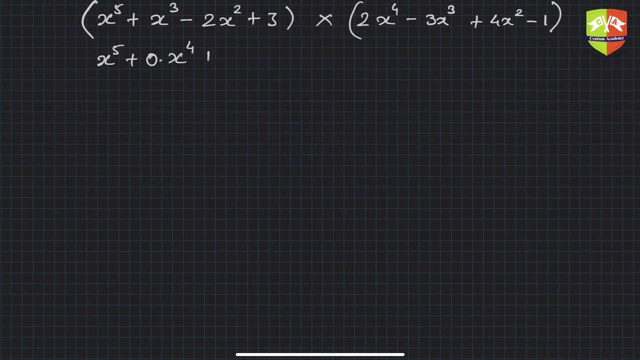 plus x, zero times x to the power four plus x to the power three minus two times x to the power four minus three x to the power four plus x to the power four minus squared, plus 0 times X plus 3, correct. and then this one is multiplied by 2x to. 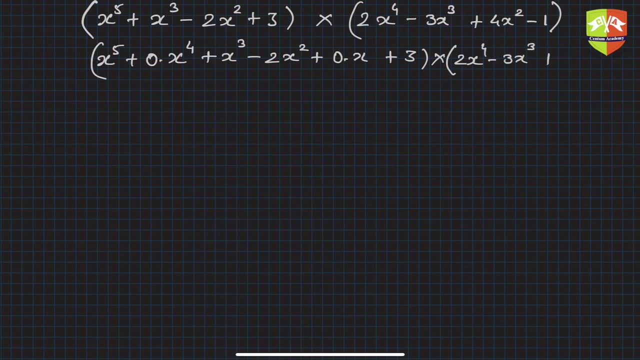 the power 4 minus 3x cubed, plus 4x squared, plus 0 times X minus 1, isn't it? now let's detach the coefficient. so detaching the coefficient, you'll get. let me start from here: 1 0 1 minus 2 0 3, correct: 1 0 1 minus 2 0 3. and the next: 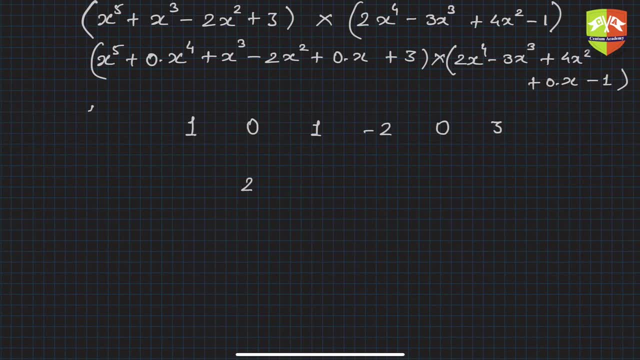 one will be simply 2 minus 3, 4, 0 minus 1. okay, now you know what to do. simply multiply like that you can. you know, if you are very, very, let's say you have practiced enough, you don't need to write in this structure. also, you can do from. 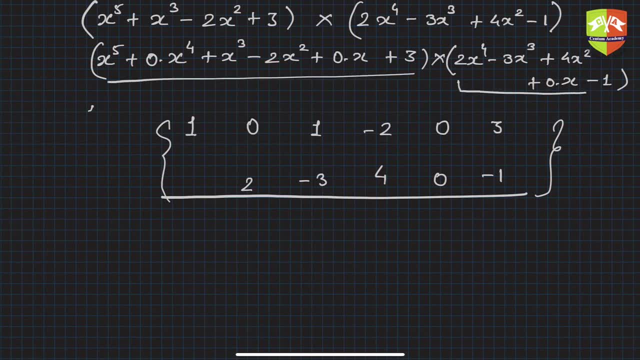 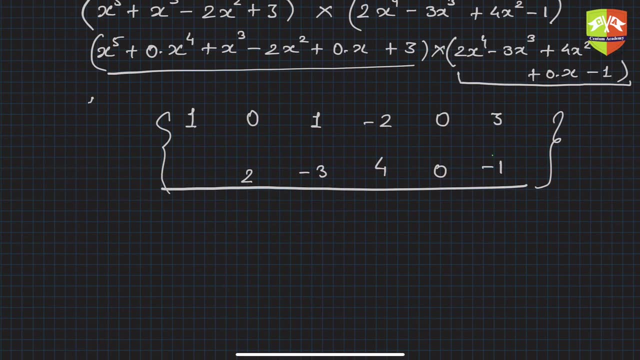 this structure also. you can do from this structure also, you can do from here itself if you, if you see, you know, if you have practiced enough from here itself, you know what to multiply when. so if you now start multiplying, so minus 1 goes to this, so it becomes minus 3, then it becomes like that. so I will do for 1. 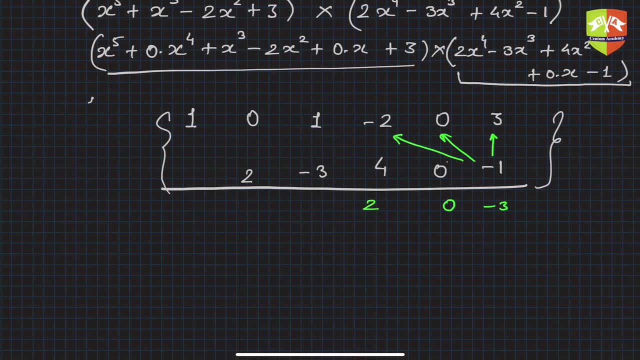 it becomes 2, it becomes minus 1, it becomes 0 and this becomes minus 1, correct? this is the first one and next one, anyways. you know, this is the first one and next one, anyways. you know this is the first one and next one, anyways. you know this is 0, all zeros. how many zeros? 6 times. 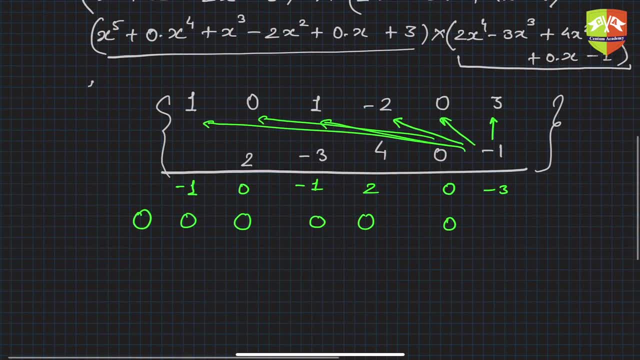 is 0 all zeros. how many zeros 6 times is 0 all zeros. how many zeros 6 times zeros? you have to just keep shifting one zeros. you have to just keep shifting one zeros. you have to just keep shifting one by one, like that. next is 4, so 4, 3s are. 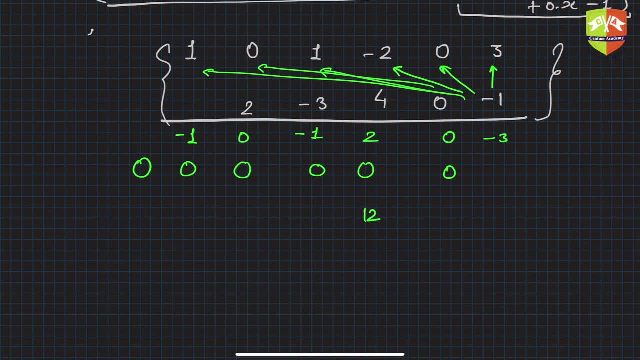 by one, like that: next is 4, so 4. 3s are by one, like that: next is 4, so 4. 3s are 12- okay, so rightful, no carry. and also 12- okay, so rightful, no carry. and also 12- okay, so rightful, no carry. and also forces are 12, 4, 0, 4 times 0: 0. so I'm forces are 12 4 0, 4 times 0 0, so I'm forces are 12 4 0, 4 times 0 0. so I'm what I'm doing. I hope you are what I'm doing. I hope you are. 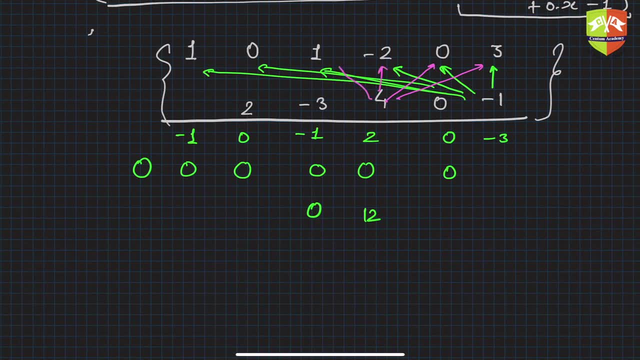 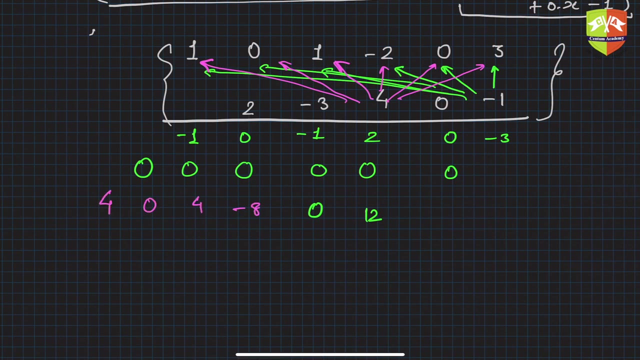 understanding. now 4, 3, 4, 0, 4 minus 2, 4, 1, 4, 0 and then finally 4, 1. i will do so. i'm writing the results now. so 12, 0 minus 8 and 4 and 0 and 4. next one will be minus 9, then 0 minus plus 6. 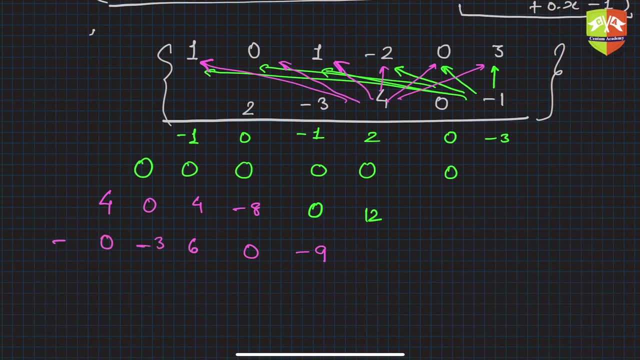 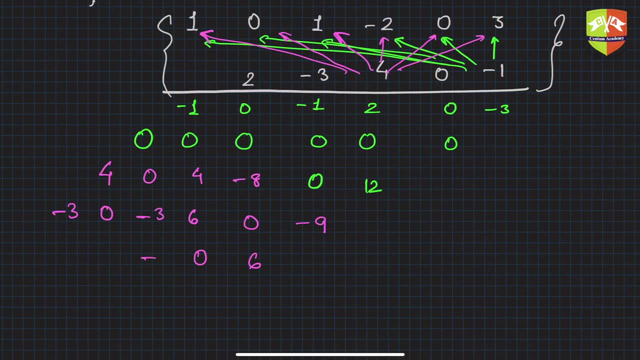 minus 3, 0 and minus 3, okay, and then finally, with 2, it is 6, 0 minus 4, then 2, 0 and 2, and then simply add, add all of them. you'll get minus 3, 0, 14, then minus 10, then minus 2, then 9. 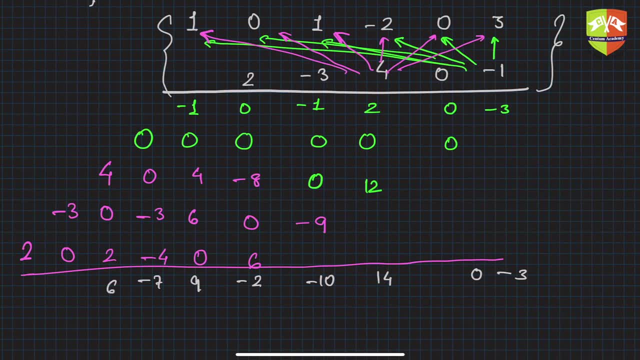 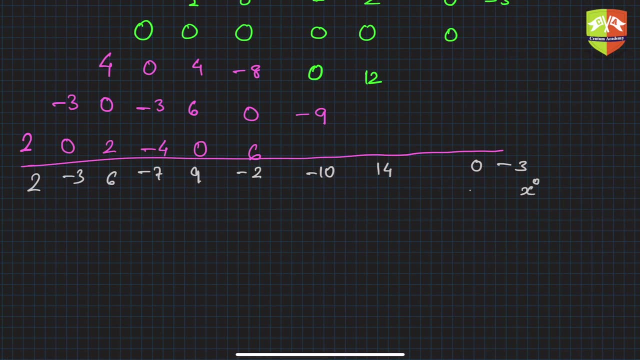 then, then, then, then, then minus 7, then 6, minus 3 and 2. okay, so, hence, now you have to just put the variable as in variable. so this is: x to the power 0, x to power 1, x to power 2, x to power 3, x to 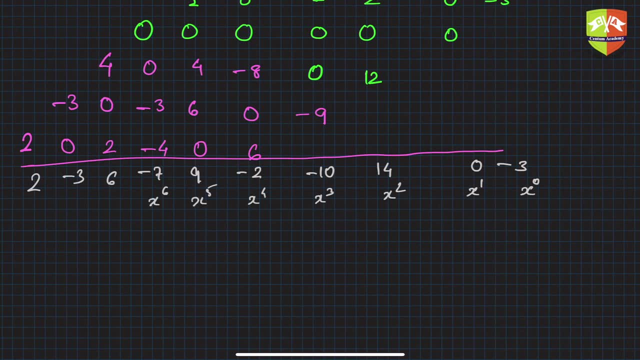 power 4 x to power 5, 6, 7, 8, 9. okay, so the answer is 2 x to the power 9, minus 3 x to the power 8, plus 6 x to the power 7. okay, so the answer is 2 x to the power 9 minus 3 x to the power 8, plus 6 x to the power 7. 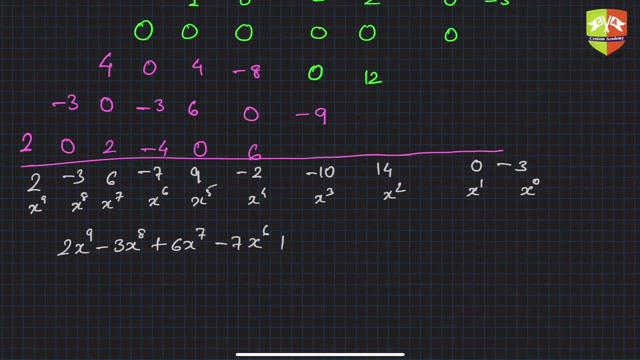 okay, so the answer is 2 x to the power, 9 minus 3 x to the power, 8 plus 6 x to the power, 7 minus 7 x to power, 6 plus 9 x, 5 minus 2 x, 4 minus 10 x cubed plus 14 x squared: 0 x n minus 3. 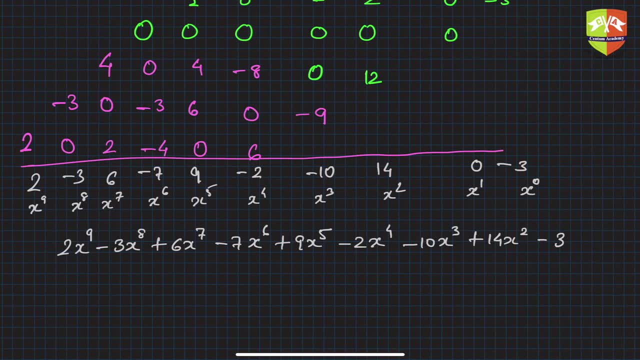 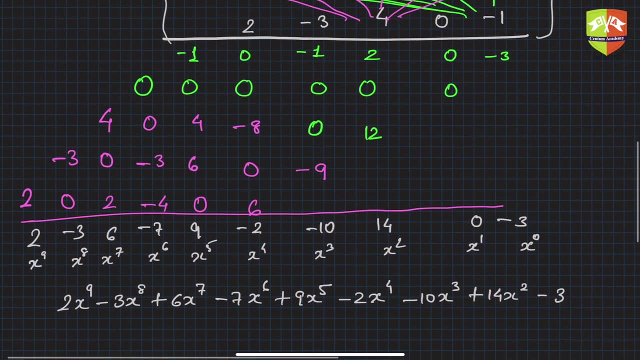 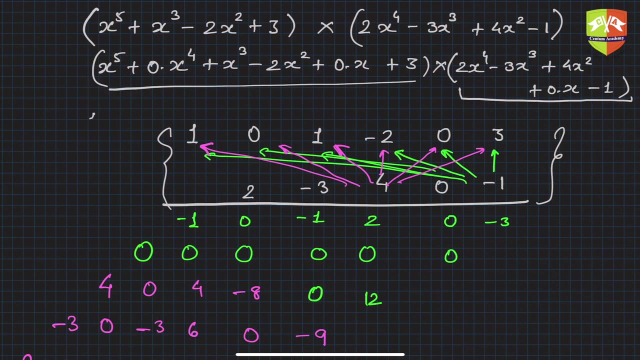 this is the product. okay, so you might be thinking that it is taking a little bit of more time while writing all of that, but you don't need to write in this format, you can do it verbally as well. okay, so that will help in. you know, multiplying two polynomials faster. so this is called. 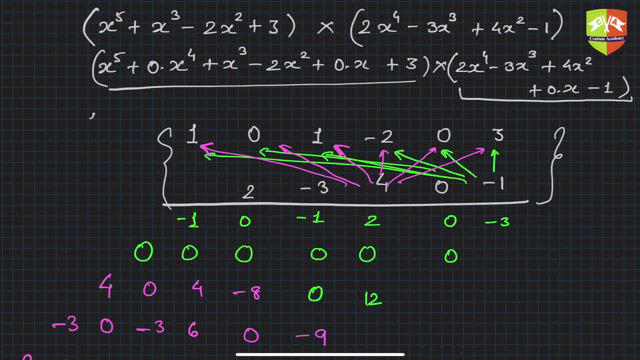 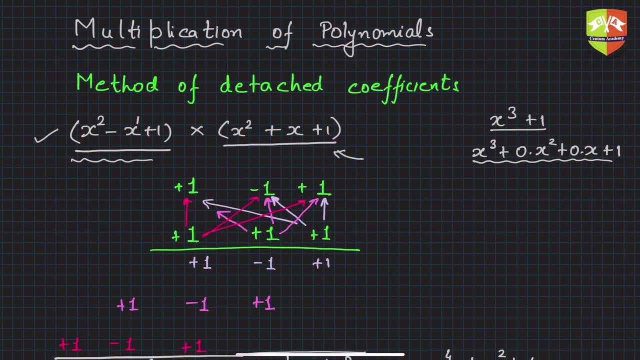 multiplication by detached coefficient. i hope you understood this process. try some more, taking some example polynomials yourself, and then try and then it will become easier to multiply bigger polynomials very, very easily.